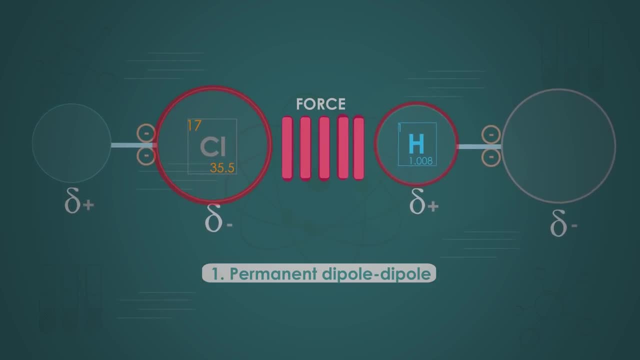 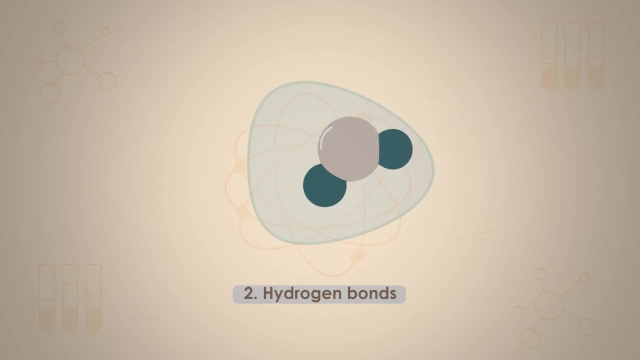 the two molecules of hydrogen chloride indicated here by the red dash. The second type of intermolecular force is the hydrogen bond. The permanent dipole in a covalent bond between a hydrogen atom and a fluorine-oxygen-or-nitrogen atom is particularly 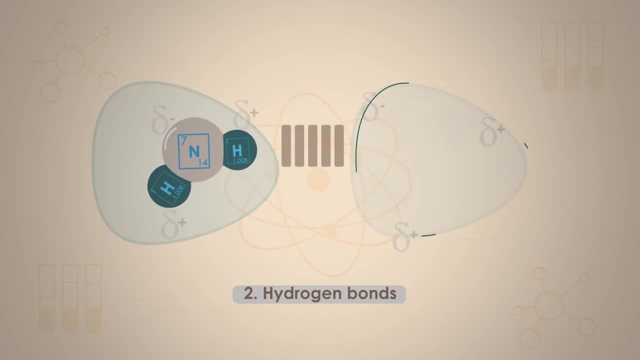 strong. Thus the attraction between the electron-deficient H-delta-positive of one molecule and the lone pair of electrons on a fluorine-oxygen-or-nitrogen atom of another molecule is much stronger than the permanent dipole-dipole attraction-match. 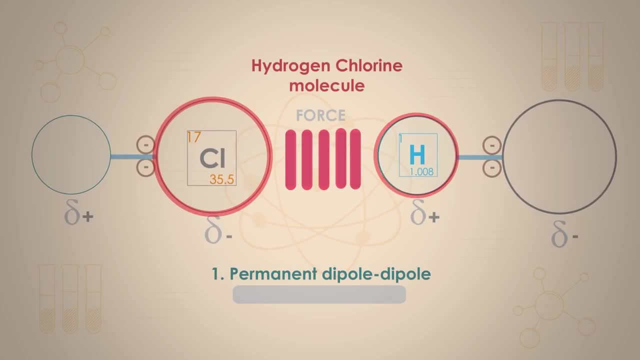 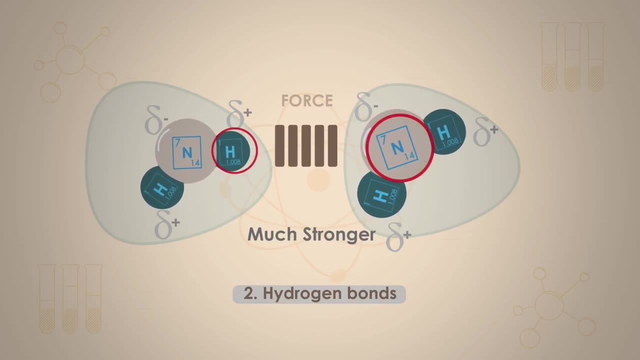 This particular type of dipole-dipole attraction between the electron-deficient H-delta-positive of one molecule and the lone pair of electrons on a fluorine-oxygen-or-nitrogen atom of another molecule is given the special name of hydrogen bond. 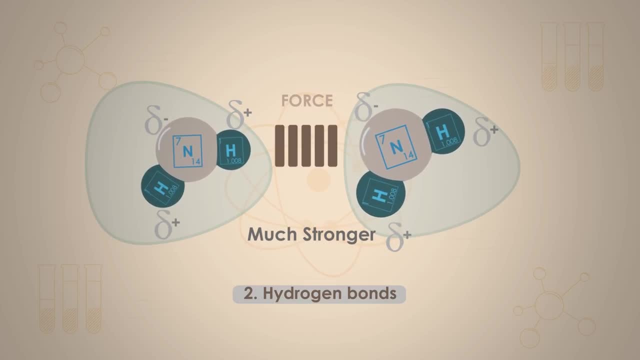 So a hydrogen bond is the attraction between the H-delta-positive of one molecule and the delta-negative on the lone pair of electrons on a fluorine-oxygen-or-nitrogen atom of another molecule. Even though a hydrogen bond has only about 5% the strength of a covalent bond. 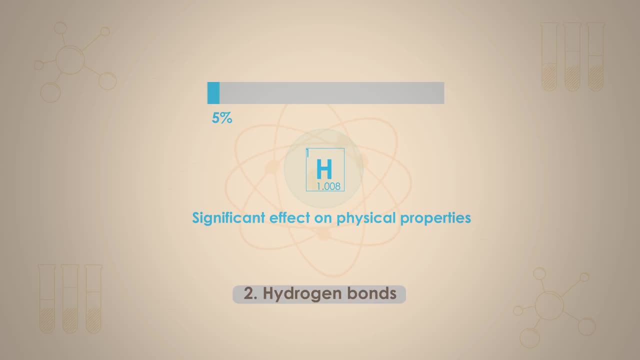 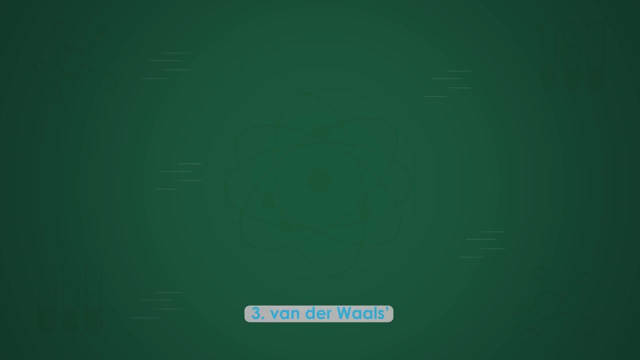 it does have a significant effect on the physical properties of compounds. For example, were it not for hydrogen bonds, both water and alcohol would be gases at room temperature and pressure. Number 3: Vandervals forces. Firstly, note the spelling of Vandervals. 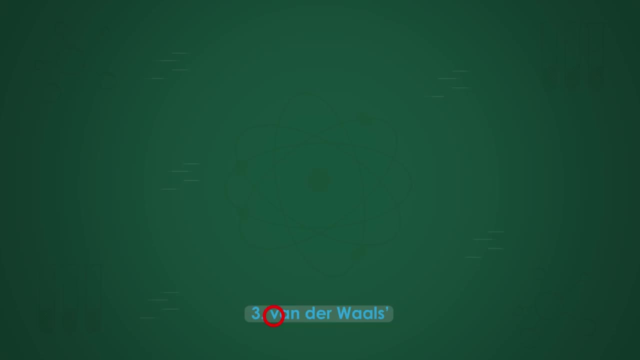 It is a lowercase v in van and the apostrophe comes after the s in vals, Vandervals, forces are induced dipole-dipole interactions. Let's look at how these arise. They arise out of movement of the electrons in the shells. If we could freeze the action at any moment in time, there would be an instantaneous dipole. 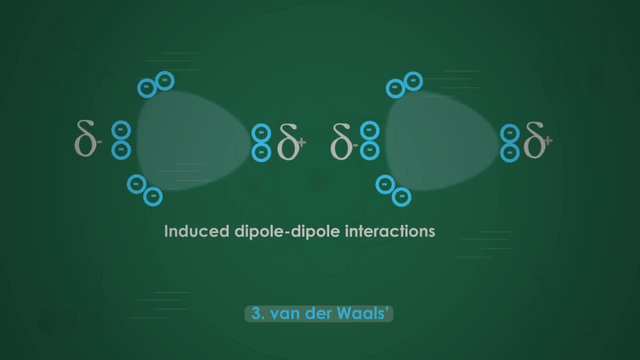 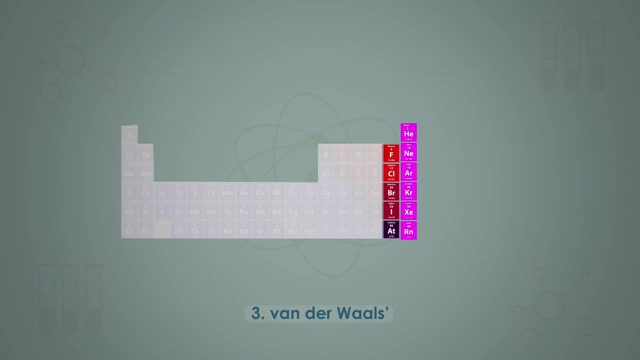 at that particular moment. These induced dipole-dipole interactions, called Vandervals forces, occur in all molecules, whether polar or not, but are the only intermolecular forces between non-polar molecules, such as the halogens and the noble gases. As the number,